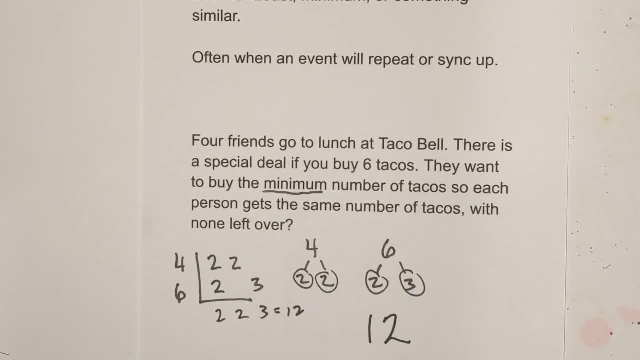 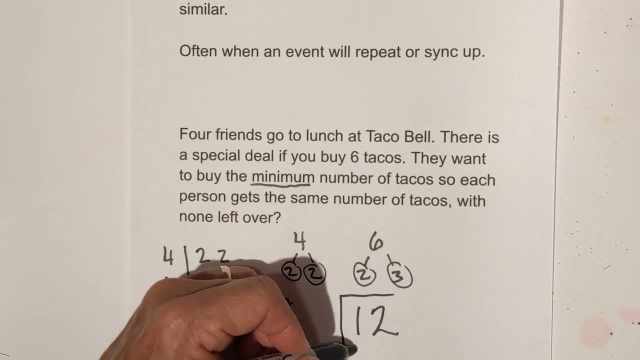 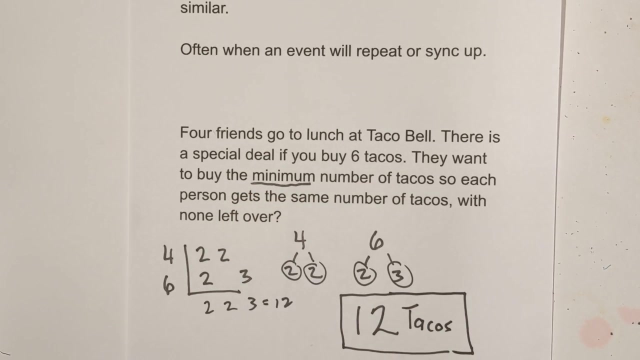 So now we know that the lowest common multiple is twelve. So what they will need to do so that everybody gets an equal amount is they need to eat. They need to buy two of the deals. Remember: They buy six tacos. They buy two of the deals. They will have twelve tacos And then each. 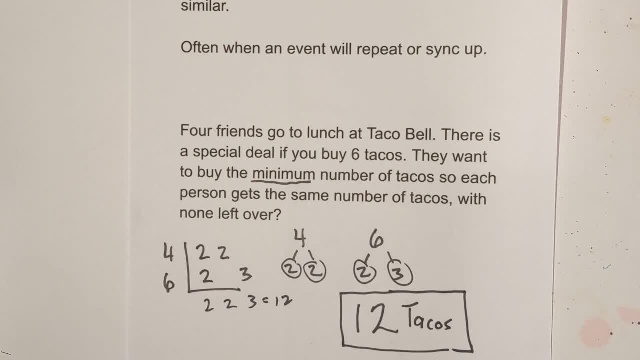 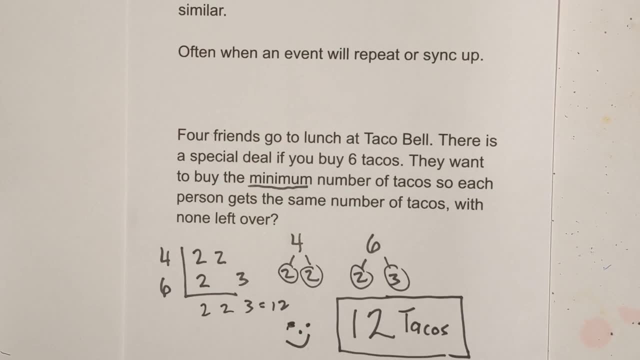 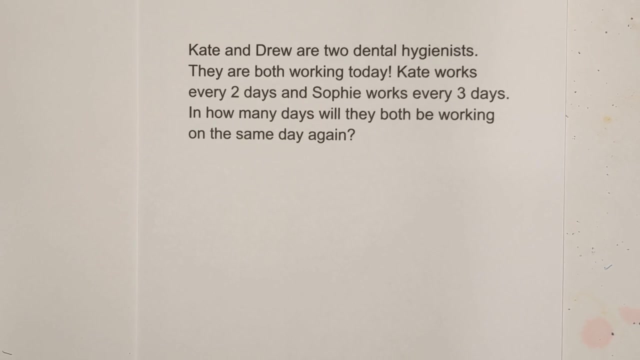 person will get three tacos And they will all go home happy. So let's have the people happy. Everyone will go home happy. Okay, let's look at another example. Okay, this example First. it uses dental hygienists. My sister was a dental hygienist for twenty. 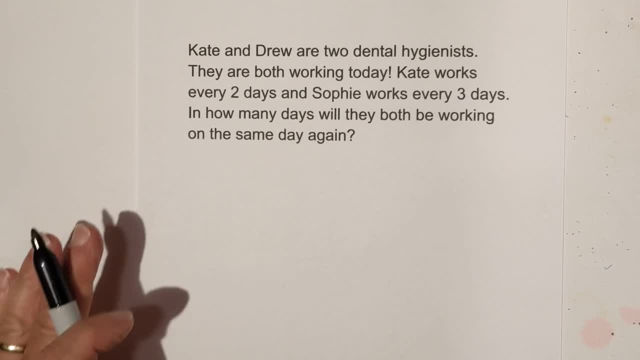 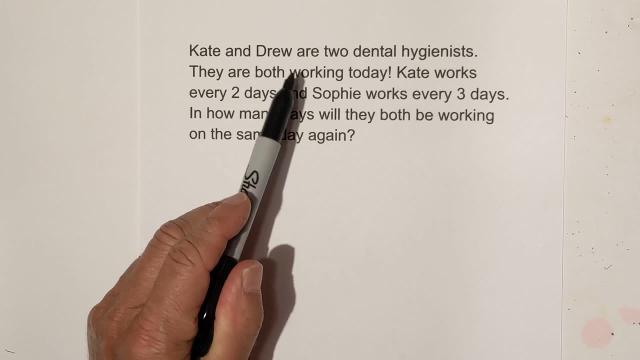 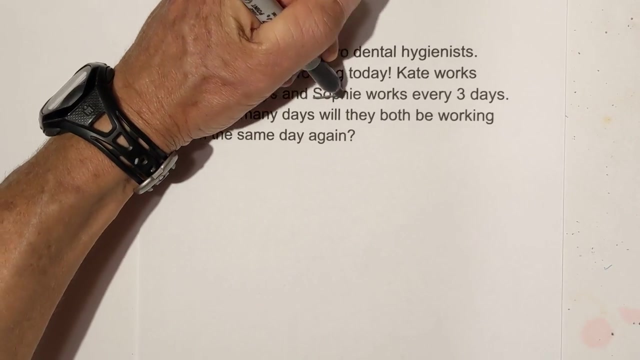 plus years And this is a LCM problem. You're kind of syncing up an event, So let's read this: Kate and Drew are two dental hygienists. They are both working today. Kate works every two days and, Excuse me A typo there, Drew. 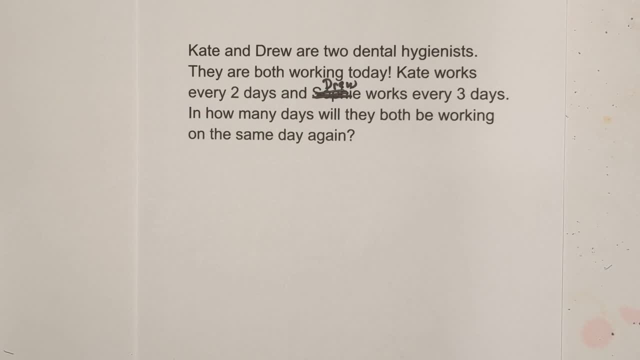 Sorry about that. Works every three days, And how many days will they both be working on the same day again? Well, let's get started. Okay, This is an LCM, because you're syncing up the minimum amount of days before they will work together. It's a minimum problem. 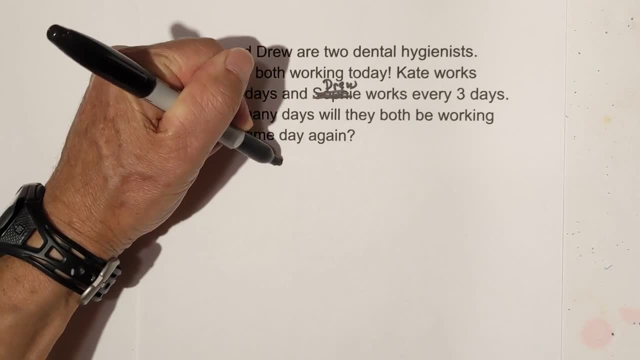 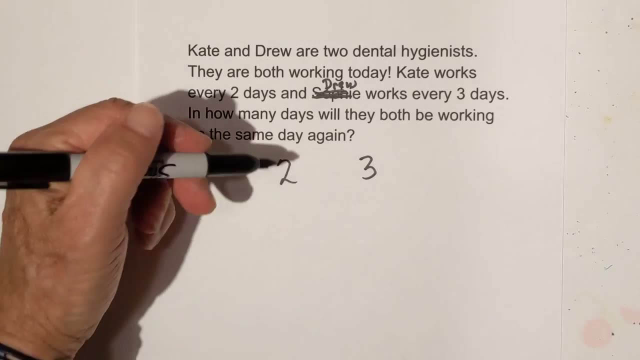 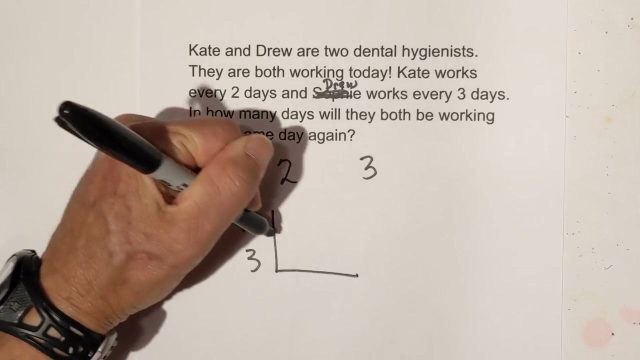 but it's just kind of disguised. Okay, So we need to find the LCM of two and three. Well, that would be fairly easy. If you use my factor tree, two is prime, Three is prime, So I'll put them in my little chart. You don't really need to do this, but I'm going to show. 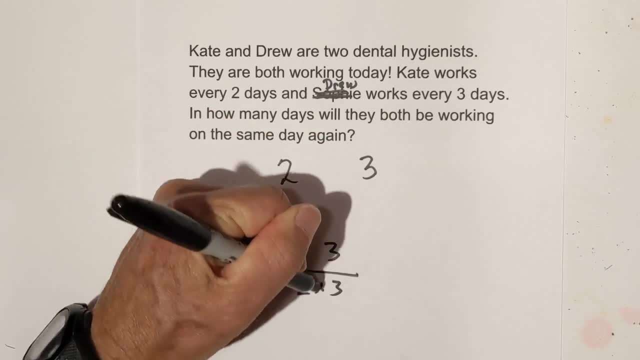 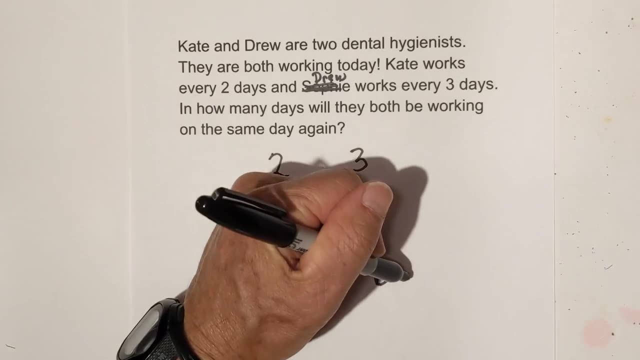 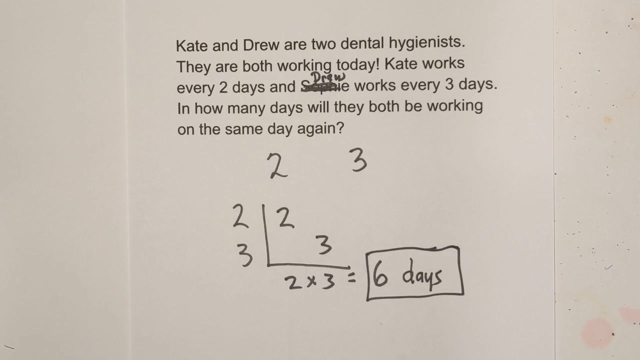 this: Bring down the two, Bring down the three, So you just multiply these together And you're done. So the LCM is six, And that tells us that in six days they will be working together once again. Okay, So that's an example of syncing up an event. I hope this was helpful. 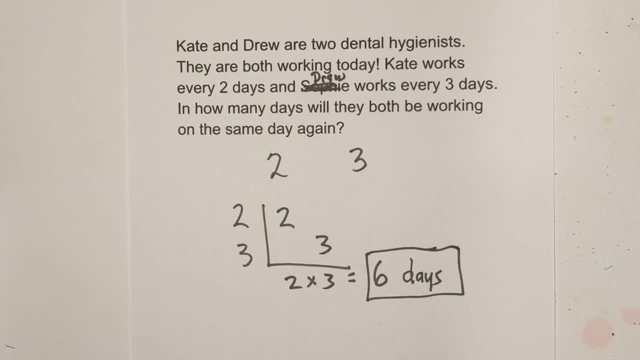 Helpful. Thanks for watching And remember. kindness multiplies kindness. Be kind to someone today.